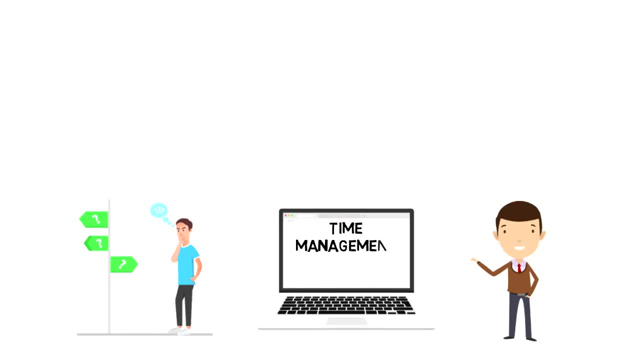 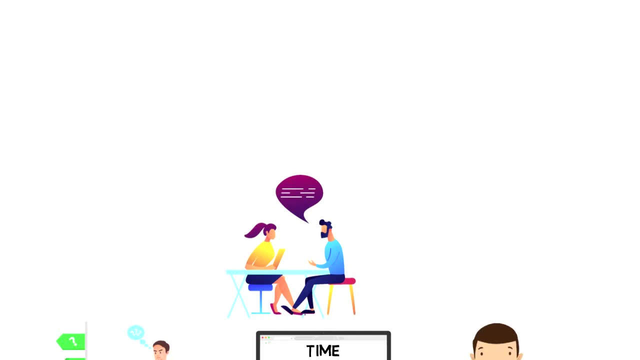 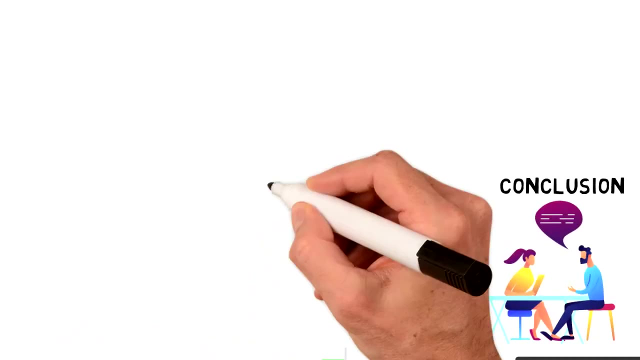 the bell icon to get updates on my latest videos about time management and productivity. Deductive reasoning, also deductive logic, is the process of reasoning from one or more statements to reach a logically certain conclusion. Thinking goes as follows: – A is equal to B, B is also equal to C, Given those two statements. 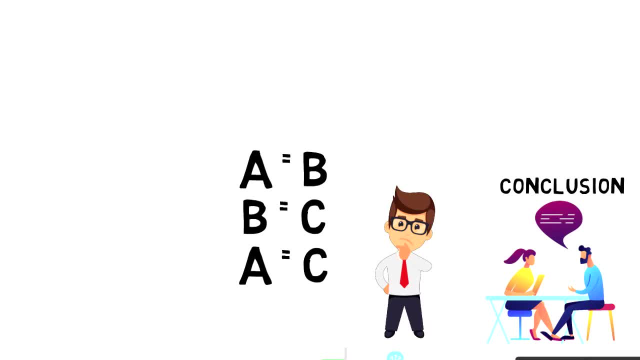 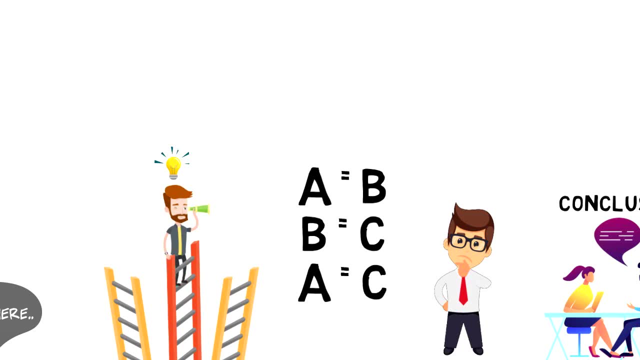 you can conclude that A is equal to C using deductive reasoning. So let's take a look at some of the examples to better understand the concept, and then we can explore how to apply it. All numbers ending with zero or five are dividable by five. The number thirty-five ends with five. So if you have more than one number, you must put it in a center on the last number of the number. If you do this, all numbers ending with zero or five are divided by five. If you have more than one number, you must put it in a center on the last number. 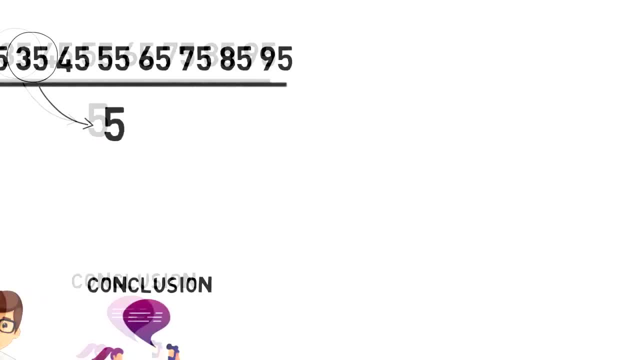 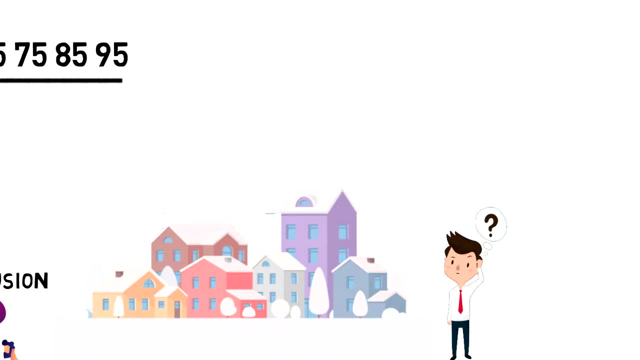 If you have more than one number, you must put it in a center on the last number. So if you have must be dividable by 5. It's dangerous to drive on icy streets. Streets are icy now, so it would be dangerous to drive on the streets. Deductive reasoning usually follows steps First. 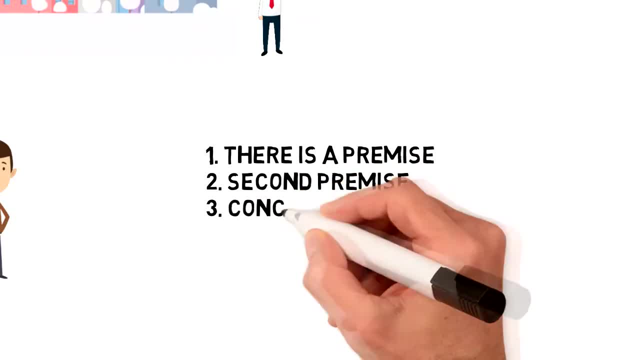 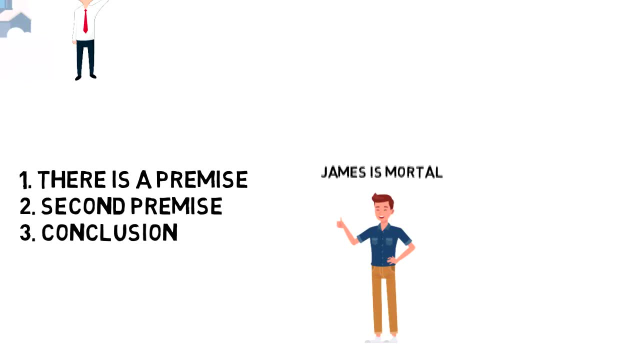 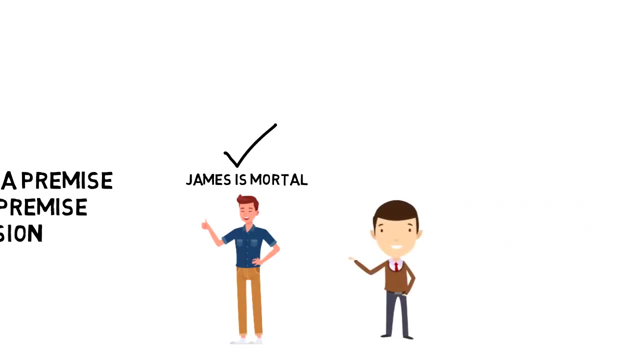 there is a premise, then a second premise and finally a conclusion. For example, all men are mortal. James is a man. therefore James is mortal. For deductive reasoning to be sound, the statements must be correct. So let's go ahead and take a look at how to apply. 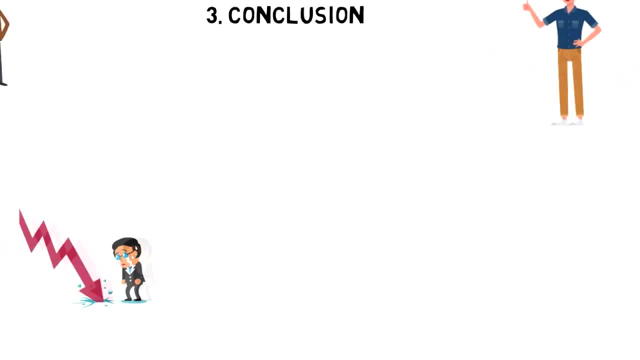 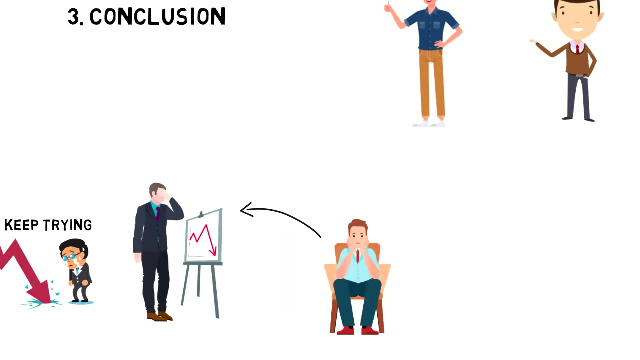 deductive reasoning to your life. Your first business idea failed. All successful entrepreneurs failed before they became successful. therefore, you should keep trying. Don't give up just because something didn't work out with the first time. Learn from your mistakes and improve for the next business venture. 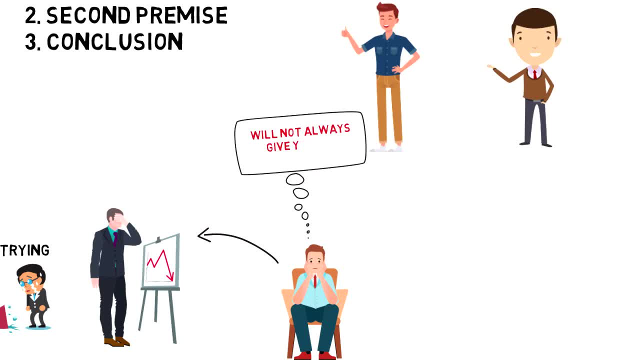 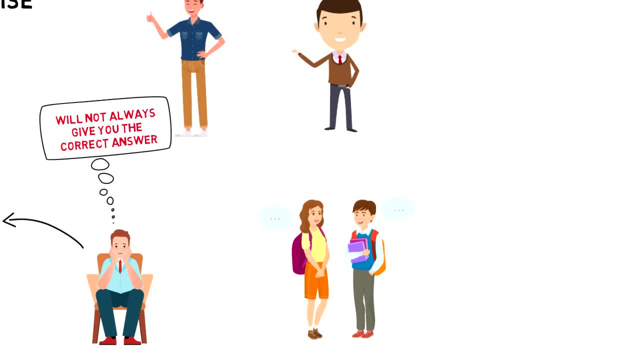 You also have to be aware that deductive reasoning will not always give you the correct answer. Consider these statements: All your college friends said that they want to make a lot of money. After college, they all went to get a job. Therefore, you have to get a job if you want. 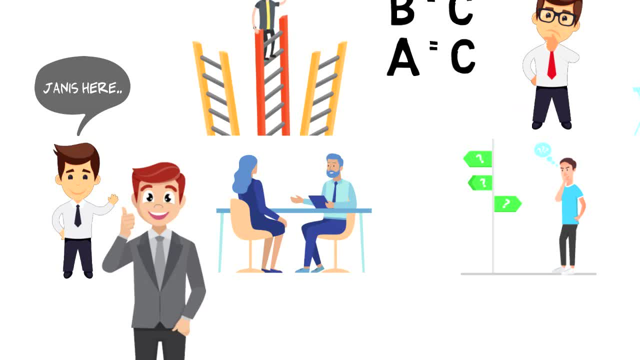 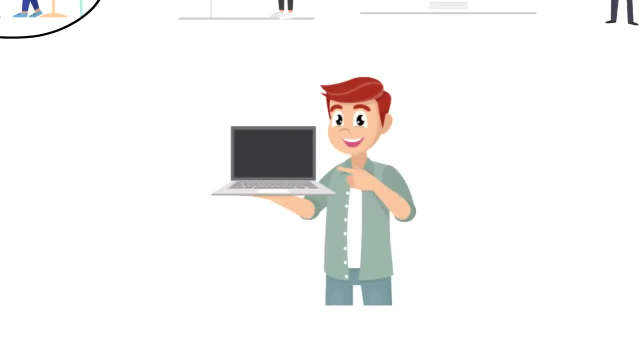 to make a lot of money. I hope that you enjoyed this video and I was able to give you a quick summary of what deductive reasoning is and how to use it. If you enjoyed this video, I would really appreciate if you could press the like button, as this will help the video reach more people. 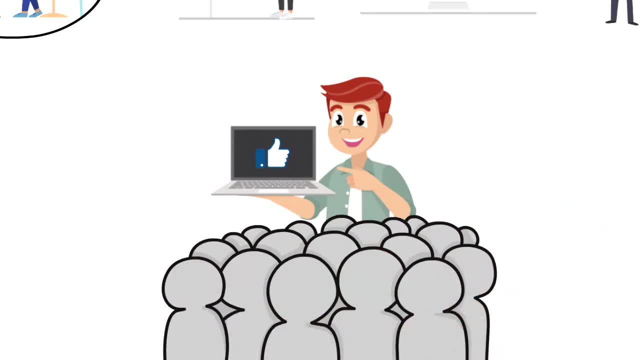 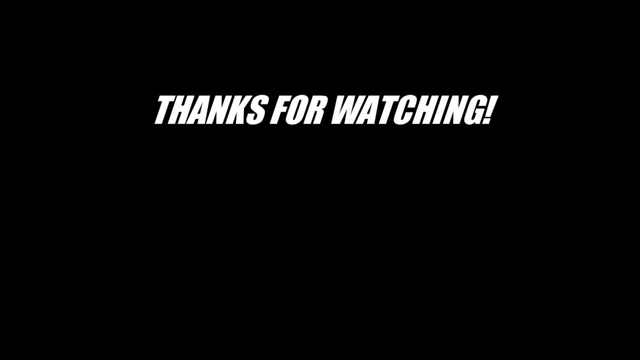 and spread the message. Thank you for watching.